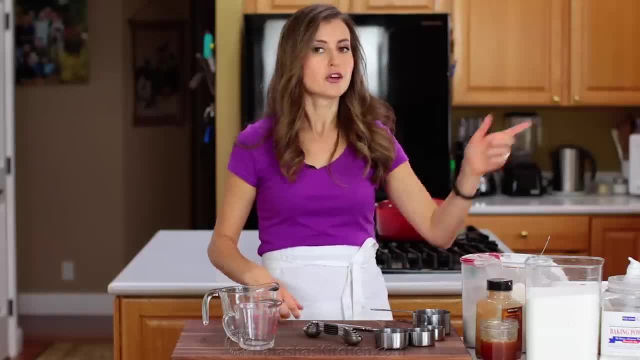 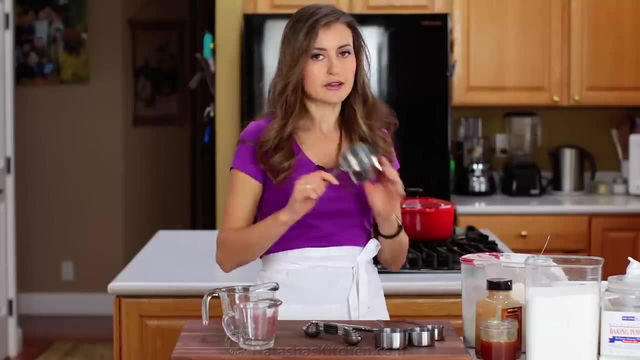 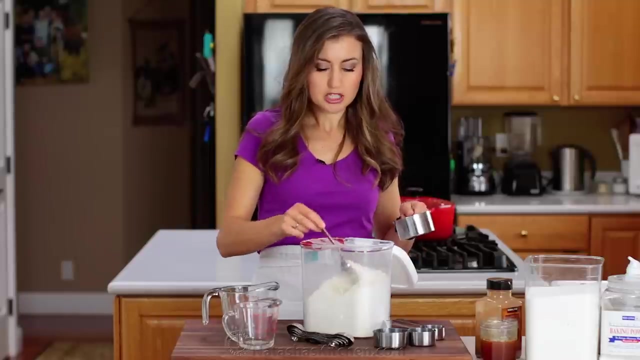 line okay, So let's get started. The first thing: the thing that gets measured incorrectly most of the time is flour, So you'll definitely need a dry ingredients measuring cup And a spoon or a scoop. The most important thing is that you've got to spoon your flour into the 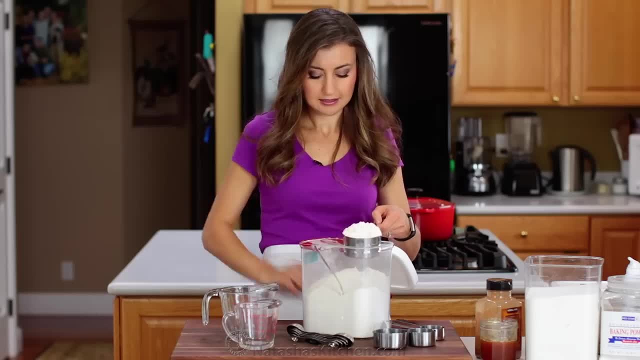 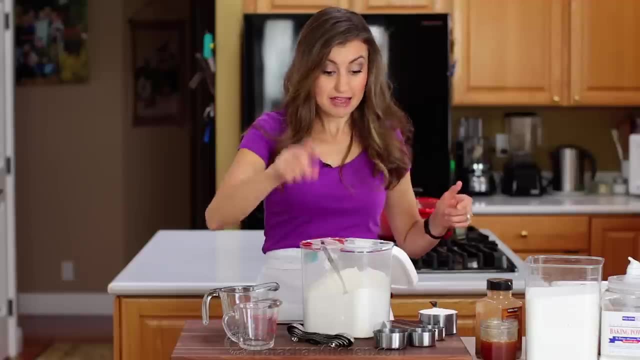 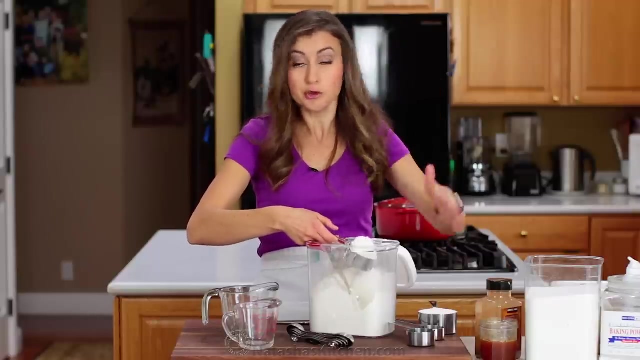 measuring cup like: so All right, And then level it off. Boom, Easy, Never, ever, just shove your measuring cup into there because it compacts the flour and you can get up to 25% too much flour. Okay, With sugar. you can dip the measuring cup into the measuring cup. You can dip the measuring 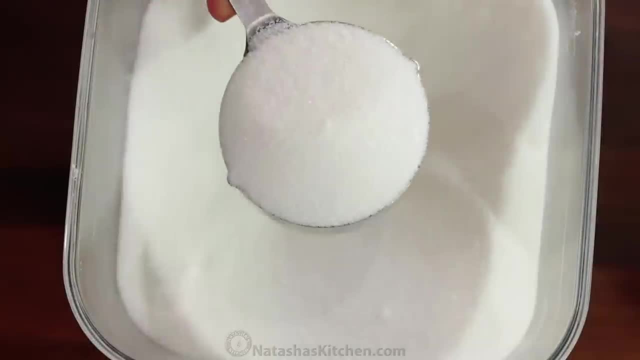 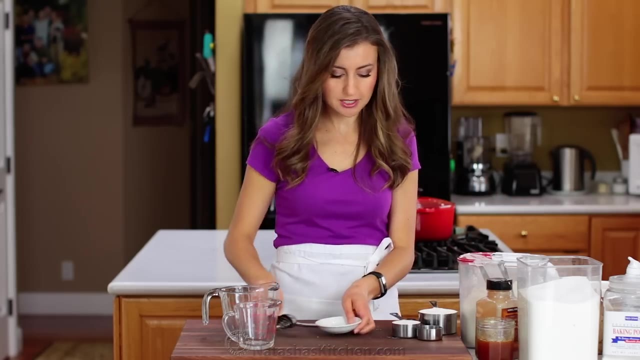 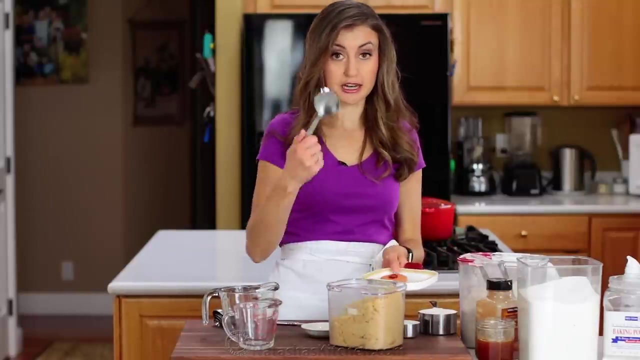 cup right into the sugar. It doesn't matter, because it's already compacted. We level off the top: Perfect measure. Now on to the brown sugar. This one's a little bit different, because a lot of recipes call for packed brown sugar. So you're going to take your measuring cup and dunk it in. 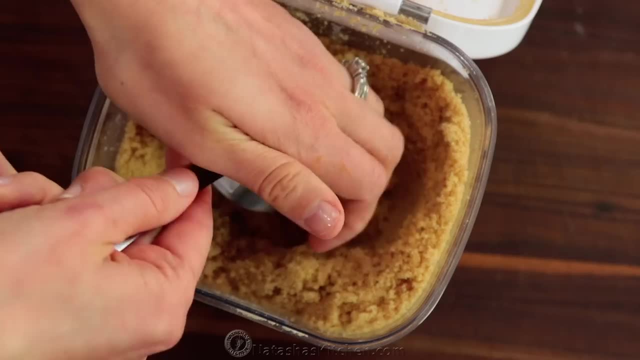 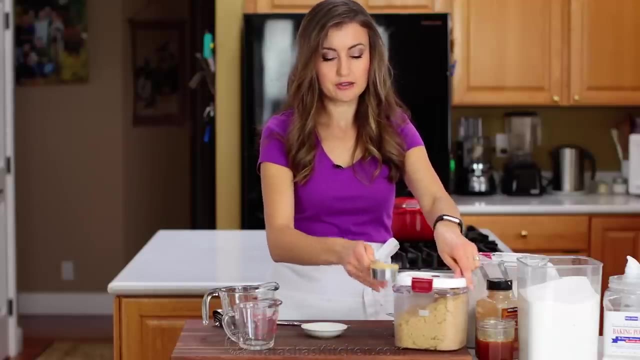 here And you're going to compact the sugar into the cup. Just push it in there, And the test of whether or not you did it right is when you invert the measuring cup into the measuring cup. You're going to put the sugar onto a plate. It'll keep its form just like that, All right. Now on to the 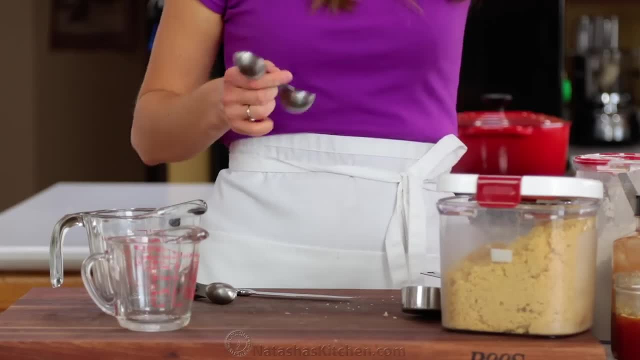 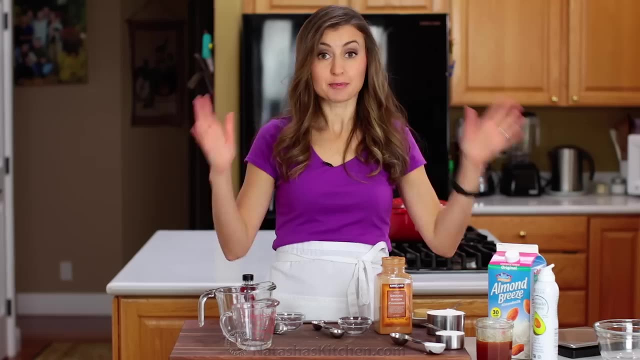 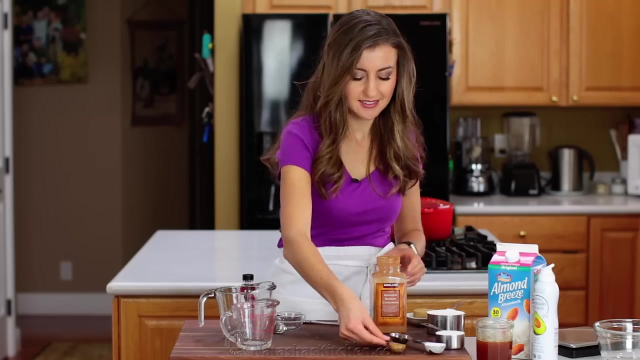 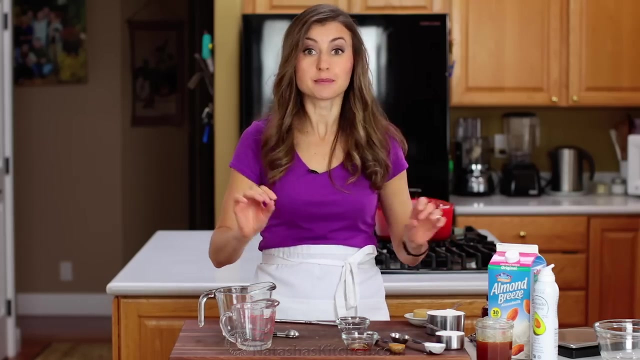 measuring spoons, So you can use these for things like baking powder. You can dip it right into there. Boop Easy Spices, same thing, Just get it in the measuring spoon and scrape. Okay. And vanilla, Just pour it till the top. All right, Now on to the liquid measuring cups. 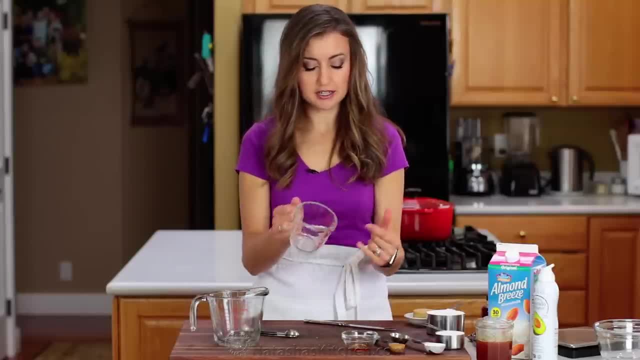 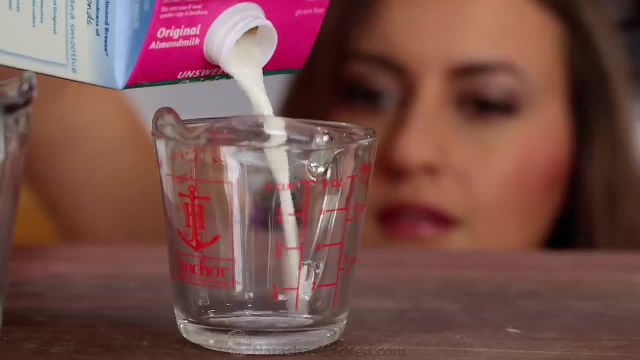 That's these guys right here. So this kind of cup you can use for, like, let's say, we have a liquidy liquid. You're going to pour that in and get down to the level of the liquid. So I want half a cup. 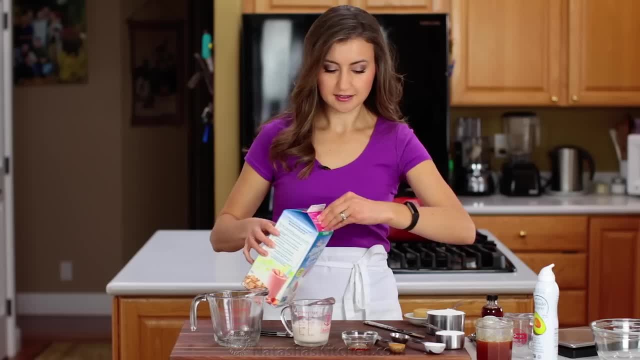 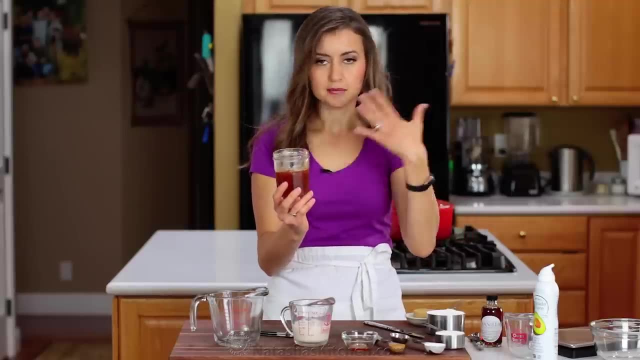 and I want to see that line right at the half cup. All right, There we go. Now, as far as if you have some sticky ingredients like honey, molasses, corn syrup, anything like that, it's a good idea to use a nonstick cup. So I'm going to use a nonstick cup. I'm going to use a nonstick cup.